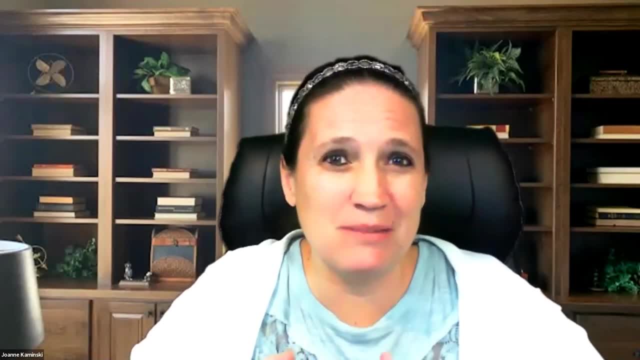 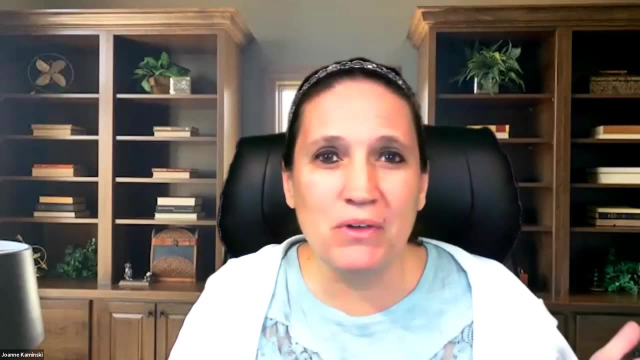 group classes, And I just want you to know that I'm just giving you this as an example of how I did it with some of my kids, And I'm giving you an example from the young side. Why? Because a lot of times people think that online tutoring can't be done with young students. We all need to be. 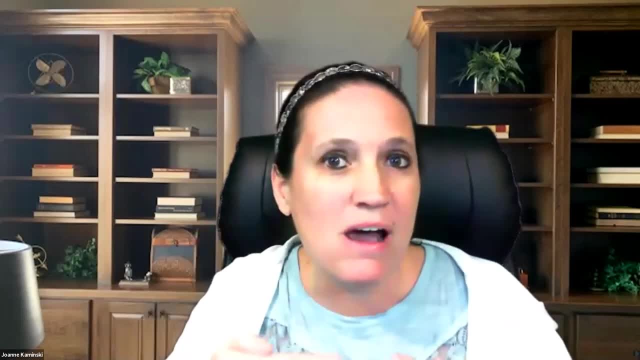 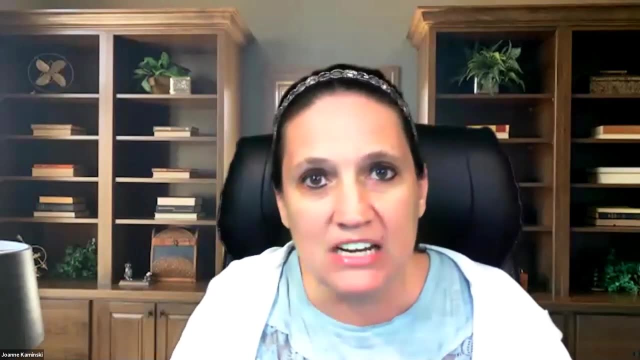 done with older students, So I want you to think about the tools that I'm going to utilize here today. How could you utilize them with your older students? Now, I know if you're not teaching reading. Raz Kids isn't going to be a tool, but how could you use the Zoom features and Google? 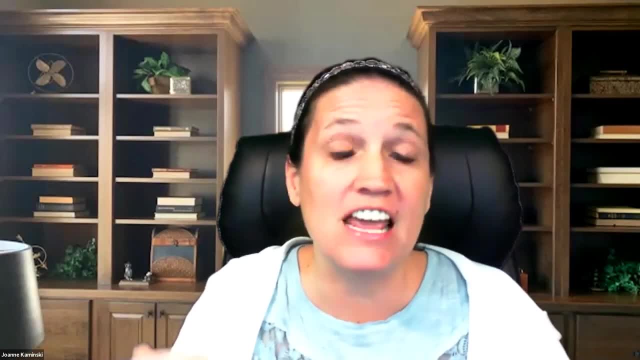 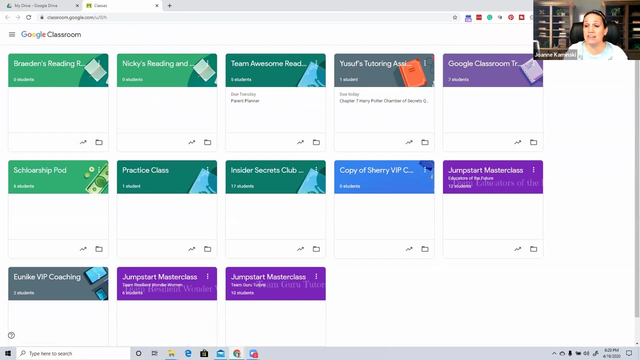 Classroom, which I'm going to show you how to use, and Book Widgets in order to be able to create your classroom and your group class. So let's take a look. I'm going to show you how I organize this specific class. So first I gave them a name, I gave them Team Awesome Readers. And, in order to create a class, 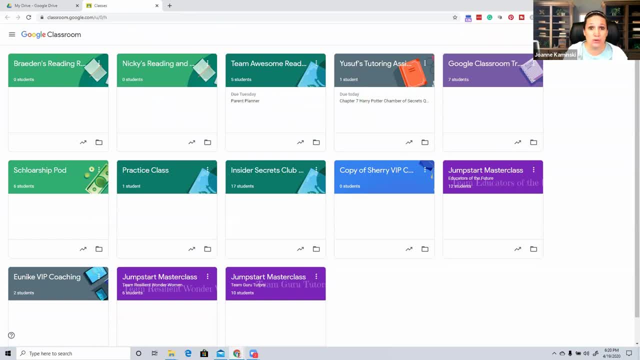 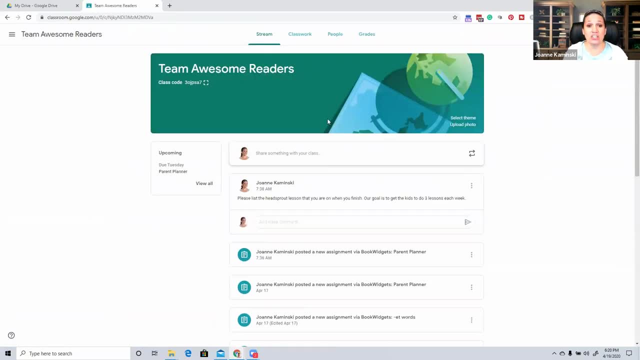 all you do is you click this little button that says Create or Join a Class, And I created a class And then I organized their classwork each week. Now I've organized this a little bit differently, So for this particular use, I'm using it as a communication tool with the parents. 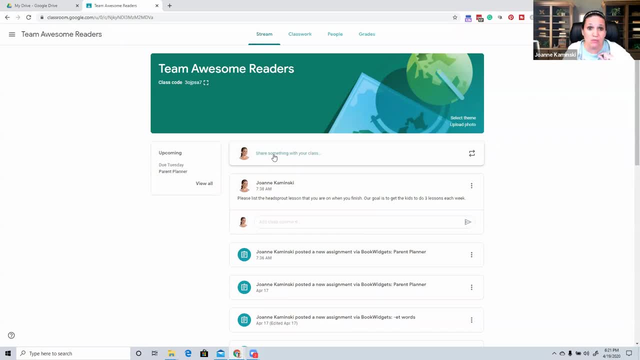 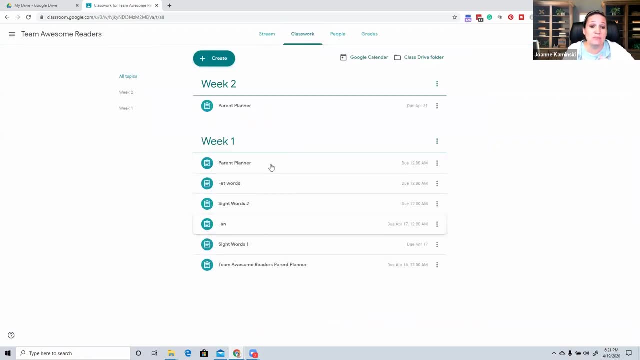 So the parents are going to be able to write in the stream. The parents are going to be able to see what the classwork is each week. So so far we have these particular assignments for week one they needed to do. And then here are the assignments for week. 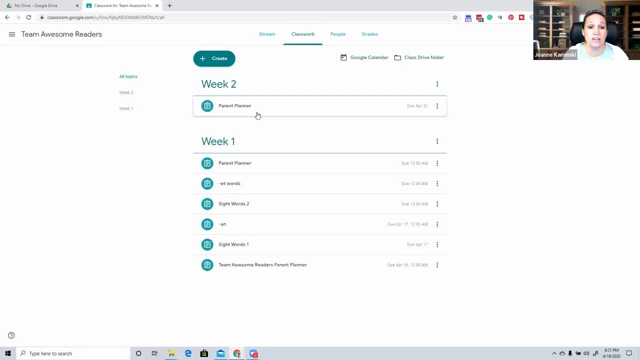 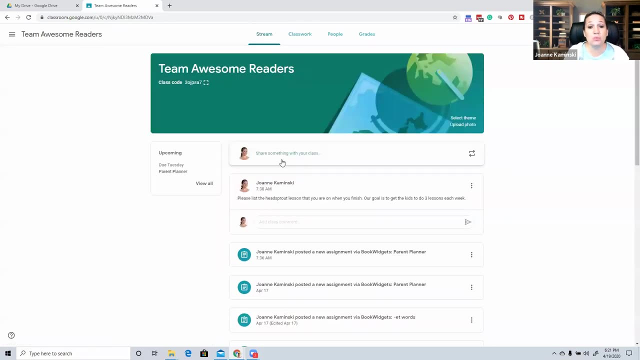 two that I'm getting started on, because this will be our second week doing it, And so what this allows us to do is just have that great way to be able to communicate. Now, if they've got any classwork that they're working on, they can actually share that right here. They can add it. 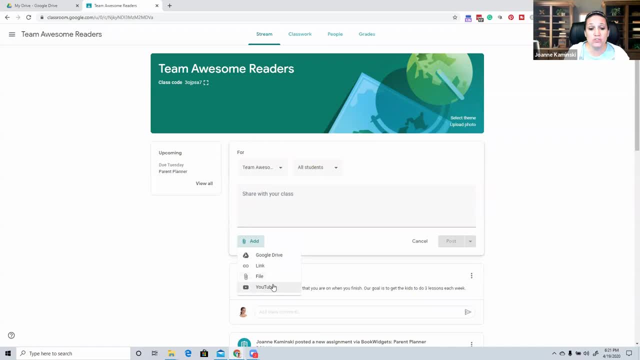 They can upload it right here, And so they can choose to share it from a file, a link they have or Google Drive, and they'll be able then to share that resource with you so that you can be able to help them. So that's one way that you could think about using it with with your older. 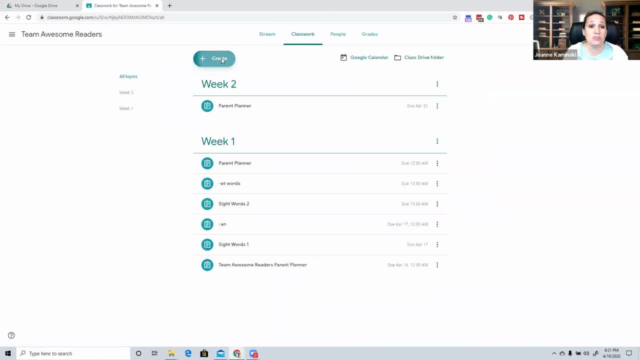 students For the classwork. you can always create an assignment right inside of here, So you can create an assignment. You can go to create a quiz immediately. if you wanted to create a quiz, You could ask a question. You could share material. I have actually uploaded a tool. 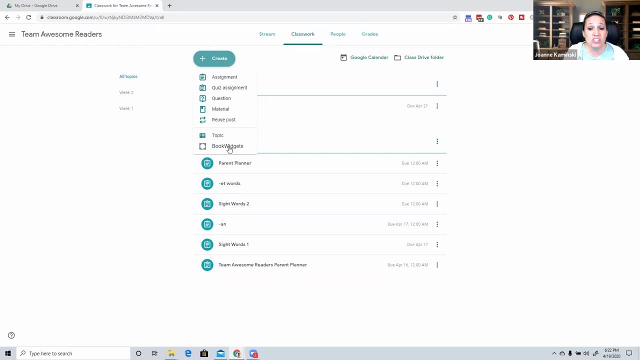 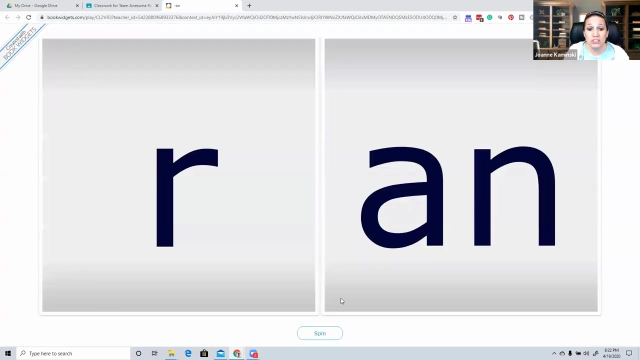 I have a tool called Book Widgets on here, And Book Widgets allows me to create tools that you're going to see like down here. So here I have some spinning words for my students to work on. So when they click on it, all they have to do is spin the wheel and read the new word that comes. So here we have o'r and ran, We spin And then here's the word. We spin again and then read a new word. So it's a fun, interesting tool. 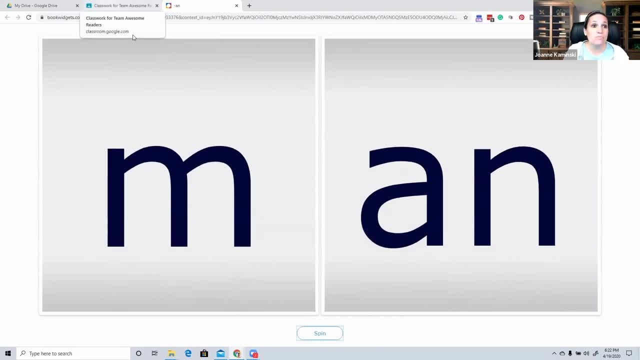 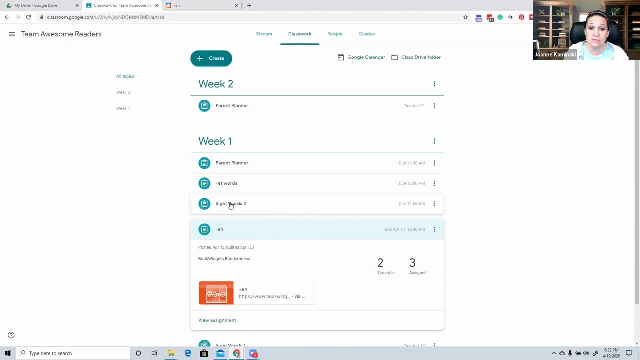 where they can click and they can spin, And these are also- I've included these- for the parents to be able to utilize with their child. We've done the same thing with sight words And I've also created a parent planner. I'm going to show you the parent planner so you can see what it. 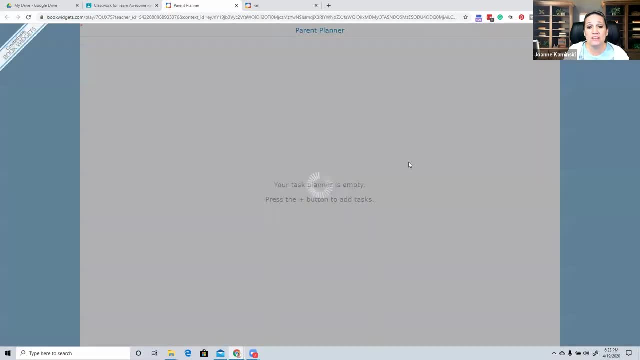 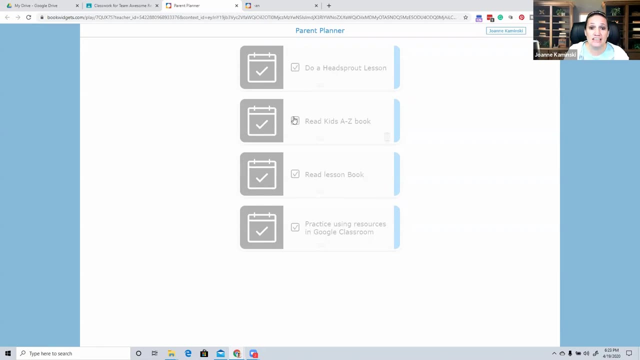 looks like With the parent planner I have organized so they know what they need to focus on every single week. And what they do on the parent planner is they're going to check if they have done each of these activities. So they check it if they've done it. So if they did a. 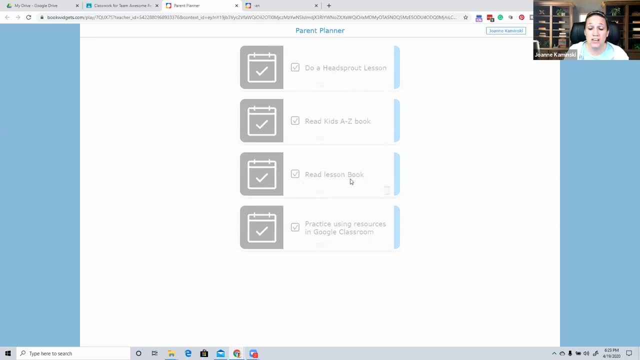 head sprout lesson check. If they read an A to Z book check, Read a lesson book check. Practice using Google Classroom resources, check And they check it off. So that's like their to-do list of what do they need to focus on specifically with their child, And I've also been using this to 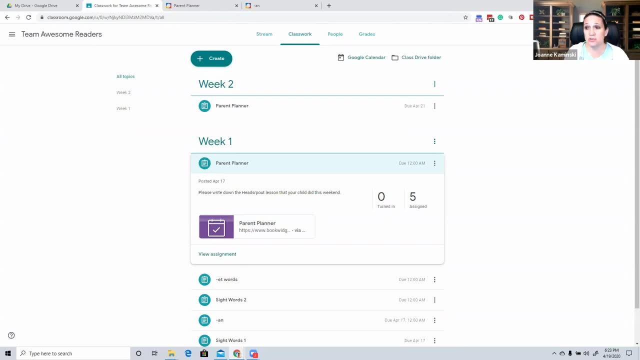 have other resources and tools that I've been able to create, And I'm just going to share this with you, And I'm going to share this with you, And I'm going to share this with you. Another classroom that I have. this is with a seven-year-old student who happens to be reading. 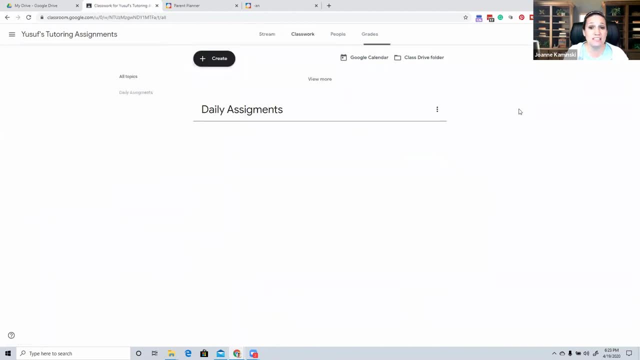 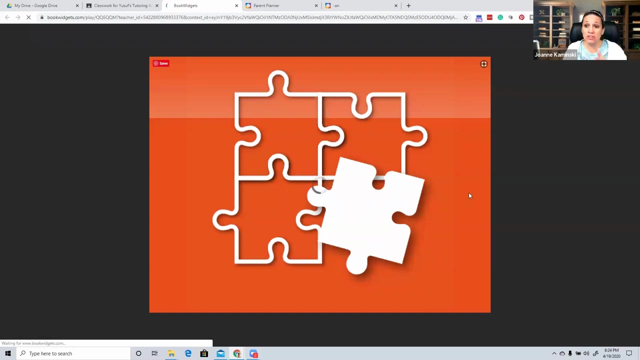 Harry Potter with me, And what I've done for him is I've created different activities, Like I've been able to create flashcards, a jigsaw puzzle- The puzzle actually is one of the images from the specific book chapter that we're reading. He has to take all of the pieces and he has to put them. 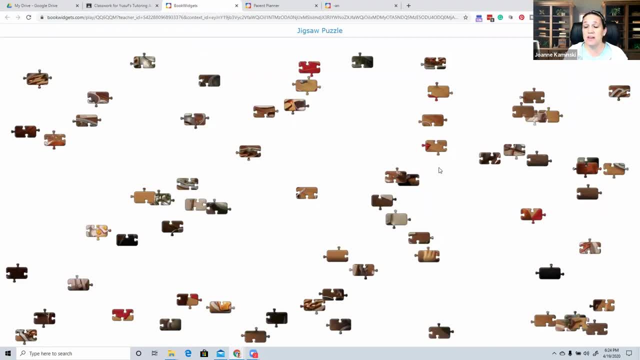 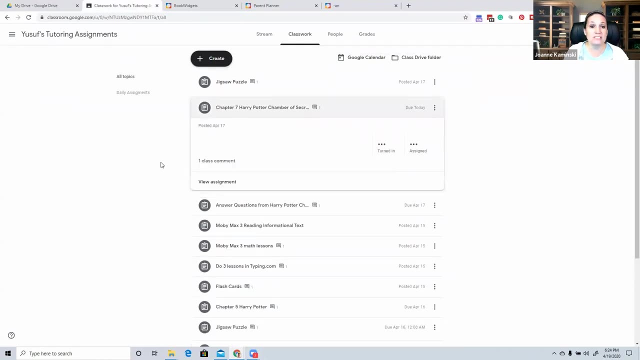 together to do the puzzle And he has to take all of the pieces and he has to put them together to do the puzzle And then he has to think about: okay, why did Ms Joanne put this particular picture in here for me to do a puzzle on? Let me take a look here. We also have I was able to create. 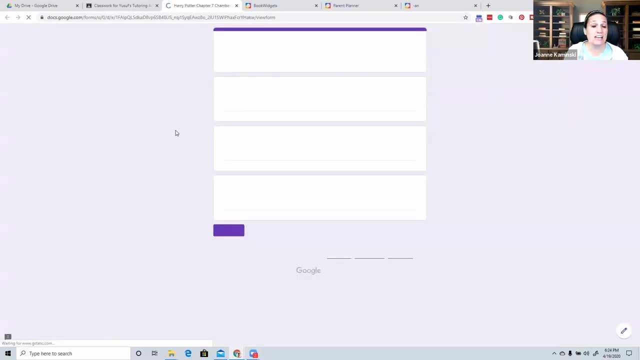 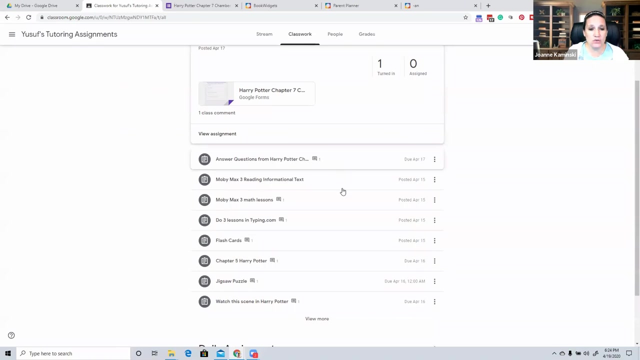 quizzes on the specific chapter that we are on. I used Google has their own quiz format, And so here he has to answer the questions. What is a mud blob? What did Harry have to do for detention? What happened while Harry was in detention? And then I also have created for him different 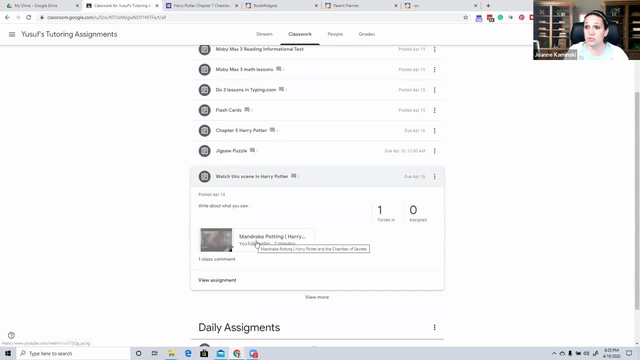 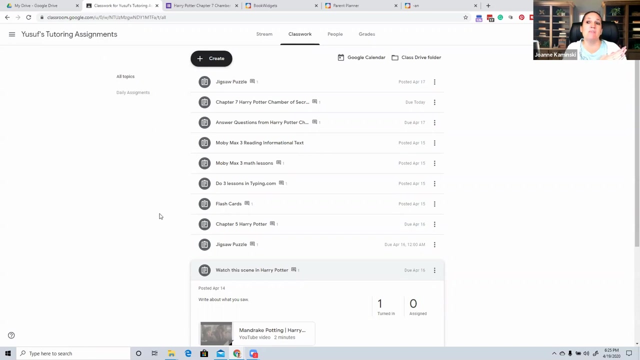 scenes that he can watch that deal with the chapter that we're reading. So this happened to be all about mandrake potting mandrakes, And so I had him watch that after we read it so he could get see. was the image he created in his mind similar to the image that was inside of the book? 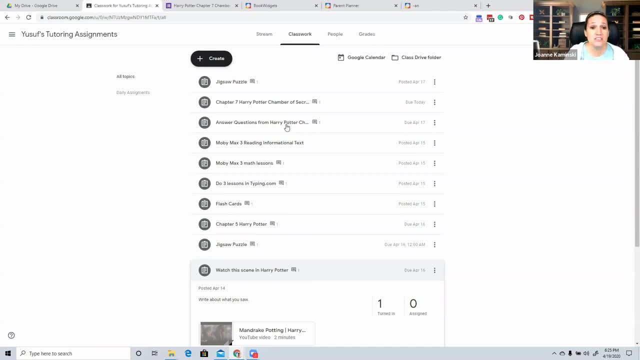 And he can compare and contrast. So there's lots of different things that you can do here, with different assignments, so that your students have work to do in between your sessions with them And it's specific to what they're working on with you. So one of the tools that I have done with my students, besides using Google- 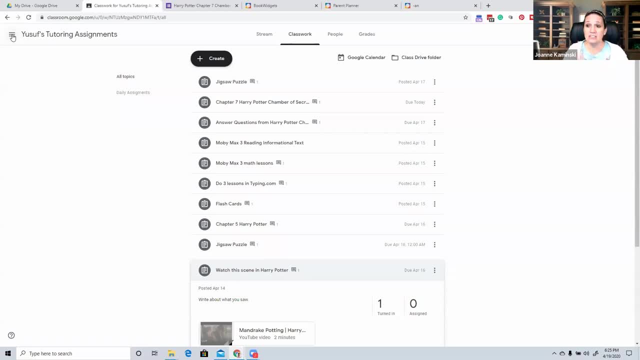 Classroom book widgets and also using the Zoom. right now I'm just using my share screen feature on Google Classroom. So I have a lot of different things that I can do here with my students And I'm going to go into my Zoom And that's what I use with my students, But I'm also going to show. 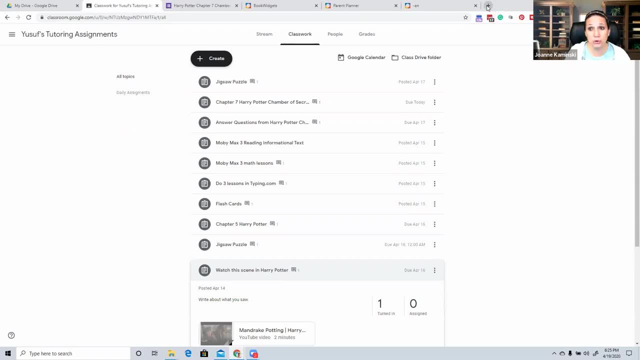 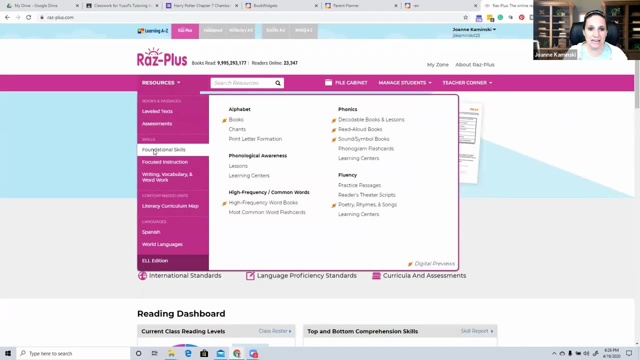 you how I use Raz Kids. So as a group I'm going to go into two places. I'm going to go to Raz Plus, I'm going to go to resources here And I'm going to click on. actually I'm going to go to level. 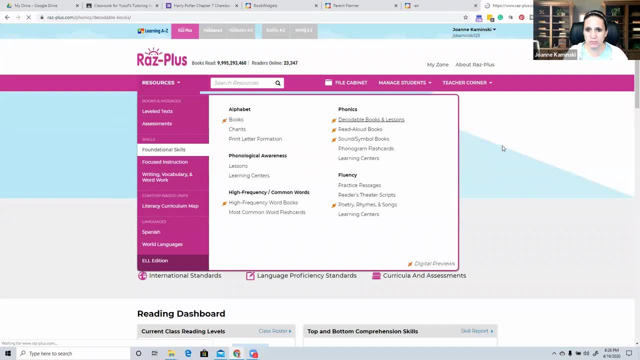 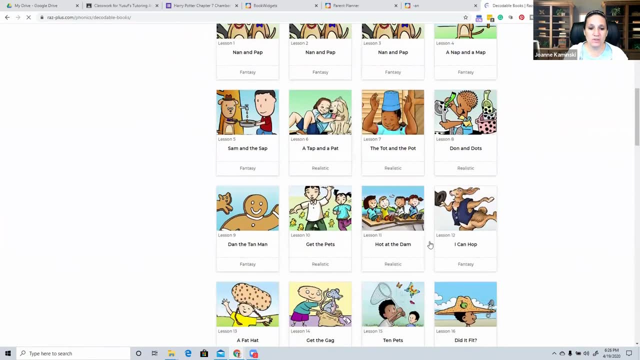 We're actually working on some decodable books, So I'm going to click on the decodable books so that their next decodable book comes on up that we're going to work on. So so far we have read Dan the Tan Man. Get the. 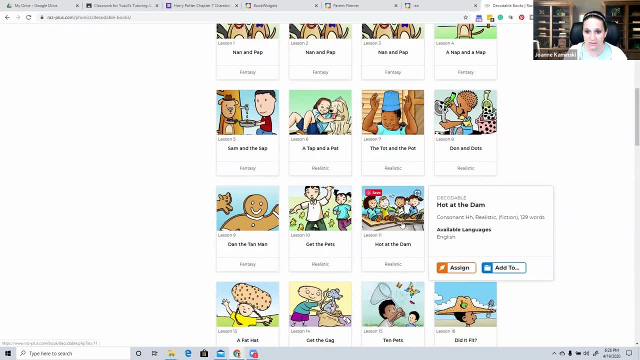 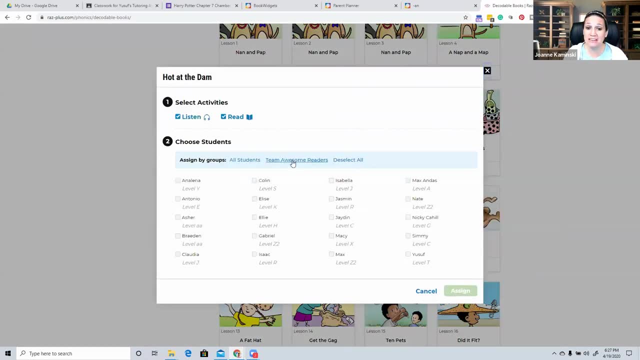 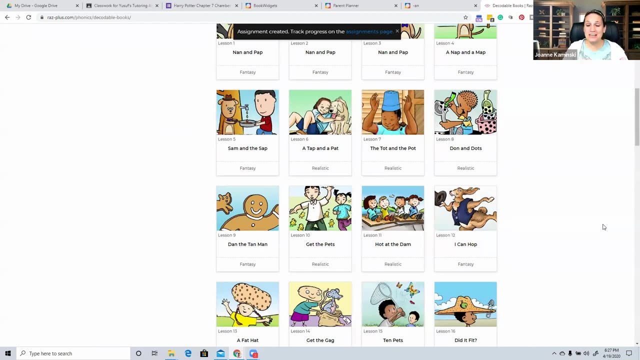 and hot at the dam So I can actually assign this book to all of my students. So I have them signed up as team awesome readers. All four of those students show on up and I can click assign and that goes right into the assignments in their kids A to Z. So let me show you what it looks like. 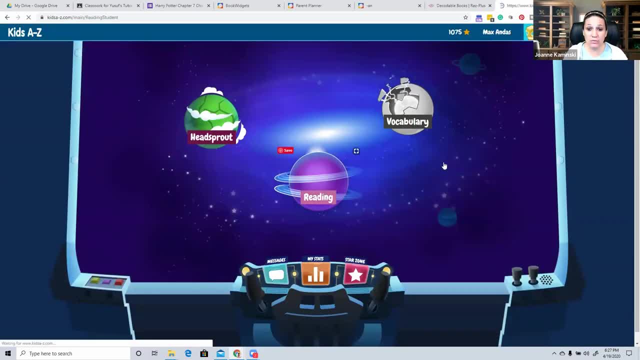 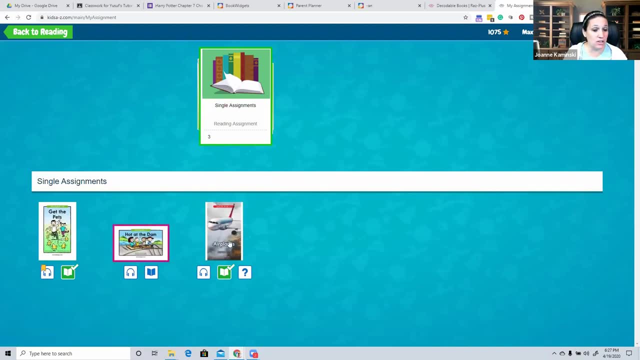 inside of kids A to Z. I'm going to click on reading here and that is going to say my assignment. So I'm going to click on my assignment and here are all of the books that we have read so far that they can continue to reread over and over again. And so these are specific assignments. If the 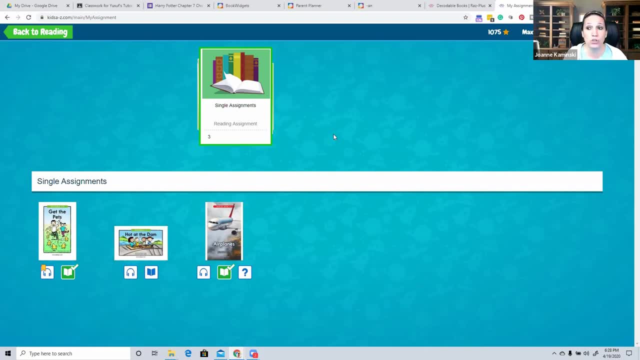 parents are going in them. they know, okay, these are the assignments that Joanne's worked on with them and they'll be able to read as practice. They can listen to the book and they can read the book. They can answer questions inside of there or they can just come on. 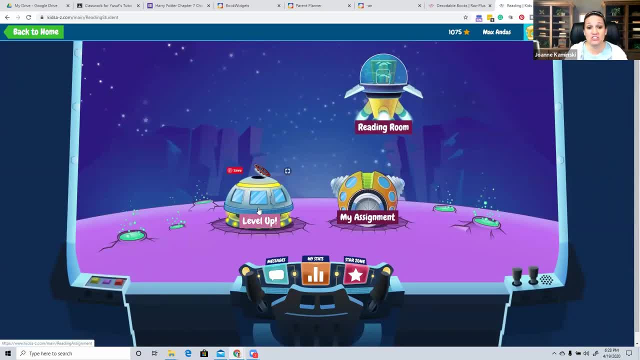 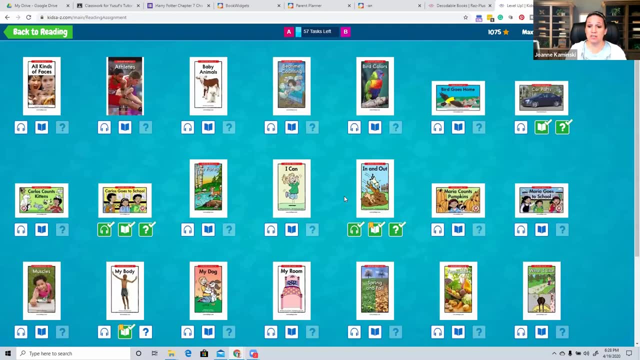 go over and choose any books that are at their level. They just go to level up and they choose any of the books that are inside of here, And these are books that they can read. I also have them right now recording the books, So when they read a book inside of here, I can listen to them. 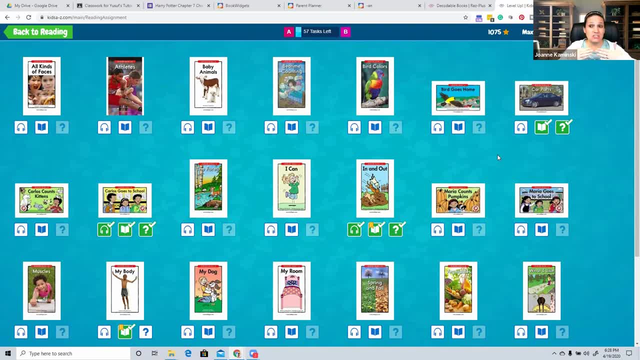 So with reading instruction, you really need to be listening to if the child is ready to move up a level. and how will you know that? Well, you have to listen to them read and see how do they do with them. So here you can have them click on a book. I'm going to go to one that this kid has already. 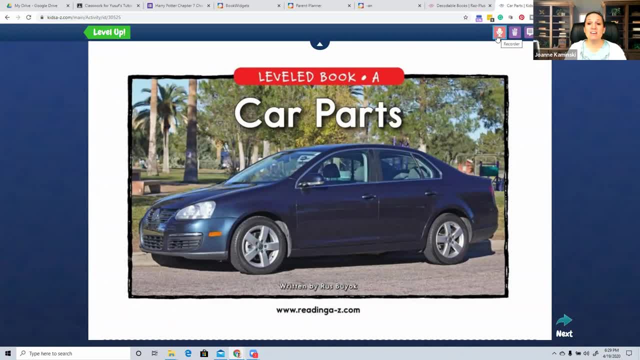 read And there's a button right here for them to record. That recording then will get sent to me so that I can listen to them read and know if it's time for them to be able to move up a level. So great tool to be able to use if you tutor reading online and you want to group your kids. 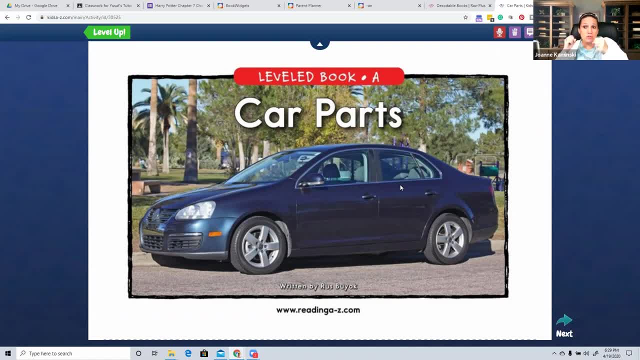 Now I've got like two sets of groups here. I've got two kids that are at a level B and I've got two kids that are at a level C. So I've got two kids that are at a level B and I've got two kids that are at a level C. 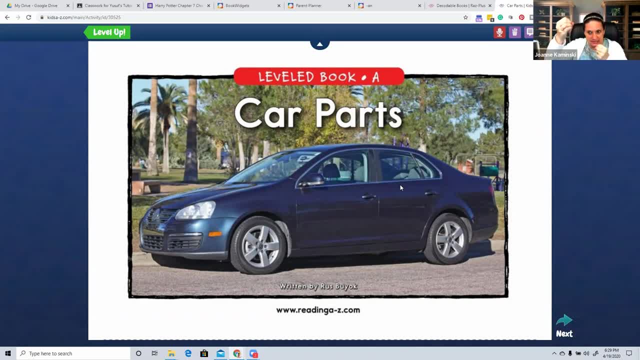 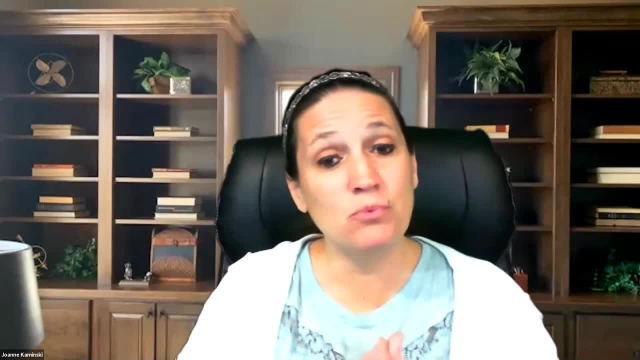 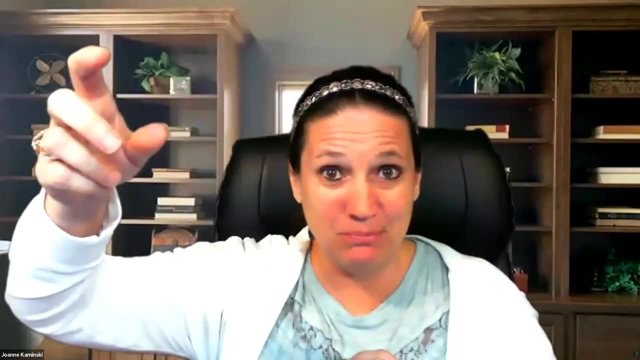 Two kids that are more at like a level C, D, And so I'm actually able to break them on up into two separate groups because of the breakout rooms. So I'm able to take one set of kids and put them into a group to practice their decodable book together, which I know that they can read pretty. 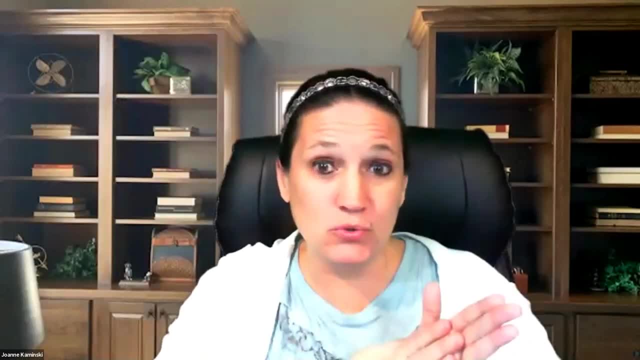 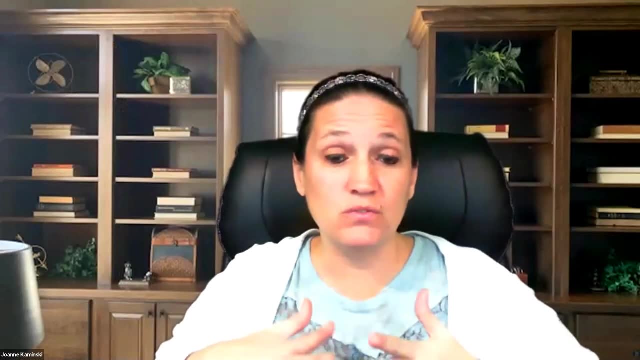 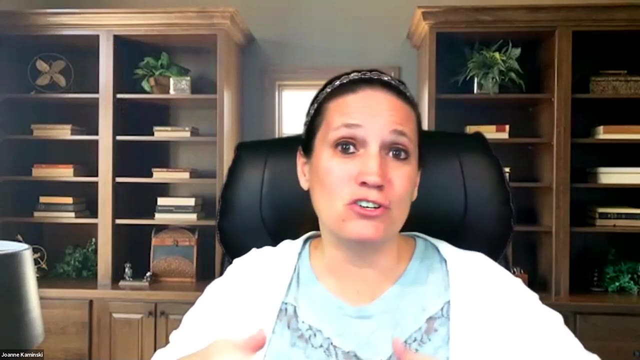 well, And then I work with the other two kids at their guided reading level. So that is how I'm able to make it work with the group class so far, And this has allowed me to give them two hours of instruction versus just the 30 minutes of instruction. So I've been able to increase. Now there may be some things. 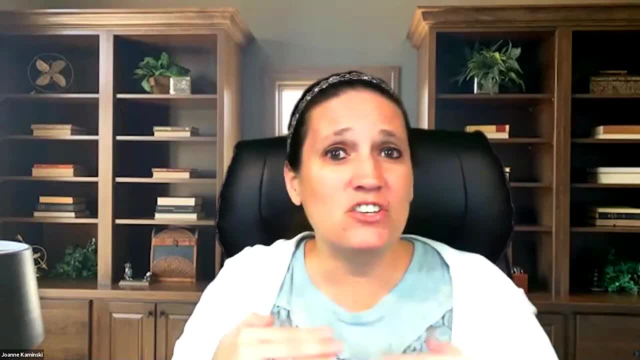 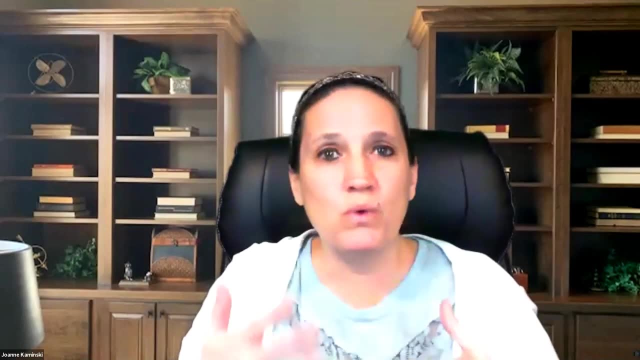 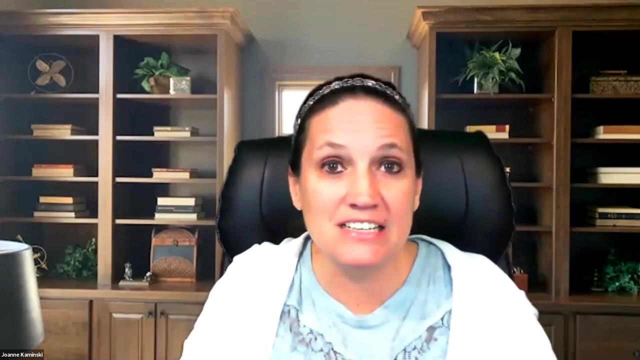 that you need to rework inside of your business. Have you thought about ways that you can help your students get more time in the subject that you have? Have you thought about different ways that you can market your business during this specific season and life circumstances that we're? 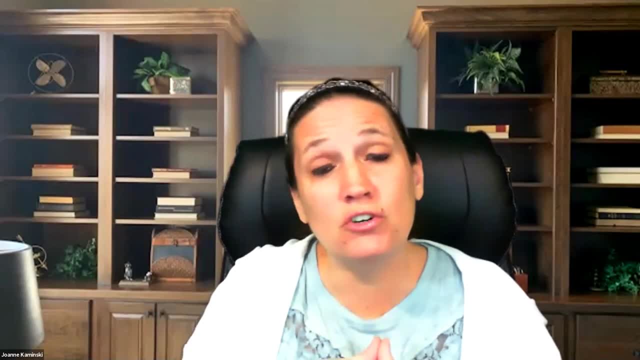 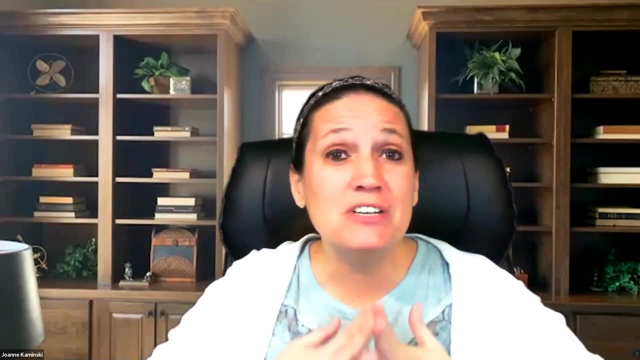 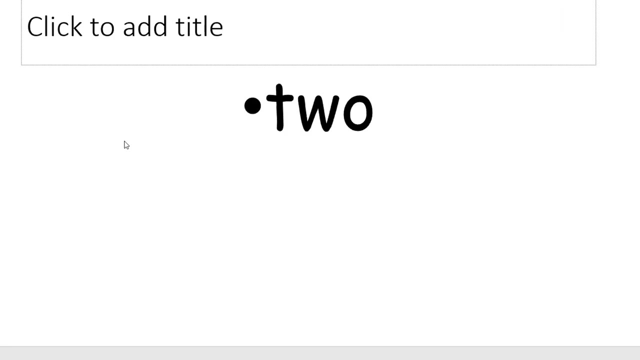 going through. If so, I would love to hear what you are doing right now. Comment below. And what I want to do right now is show you specifically what it looks like in my classroom with my students. No, Okay, This word let's see. Oh, Antonio thinks he knows it. What is it, Antonio? 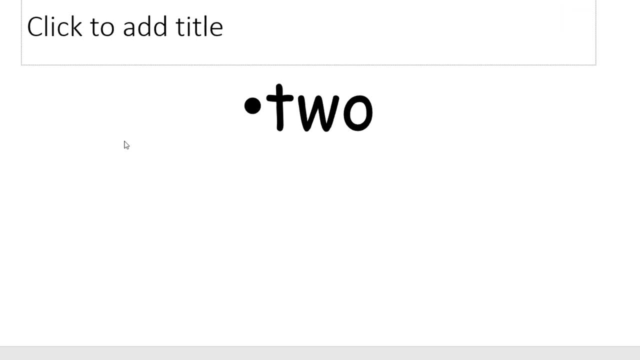 Two, Two. Shake your head if you think that's right, or you don't think it's right, Right, That's right, Yes, Good, All right, Let's try this one. Who knows this one? Oh, you think you know this one, Jayden. 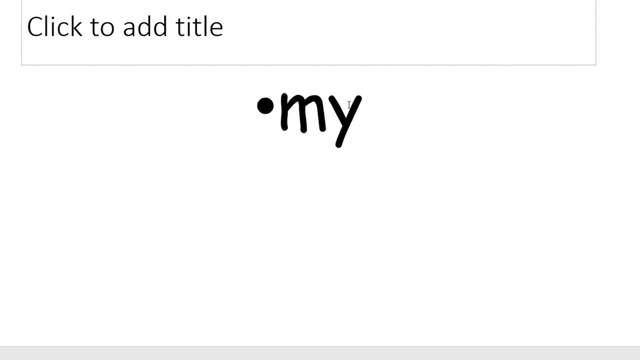 Me Almost. My Yes, my Good job. All right, Let's see if we know this one, Antonio. Three, You got it. Three it is. Let's try this one. Max, you want to give this one a shot? 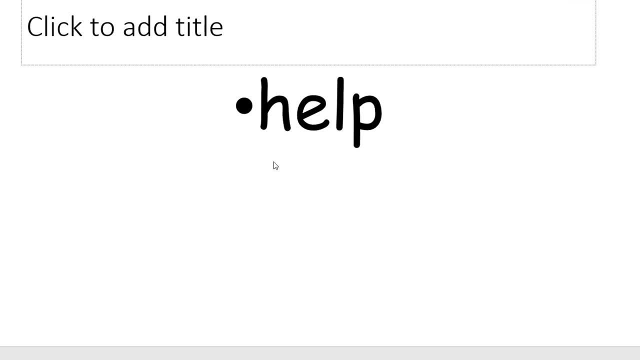 So here I'm showing you my students. I'm going to give this one a shot. I'm showing my students the sight words and they're able to read them, figure them out and do the sight word work that we usually do at the beginning of the lesson, but as a whole class. 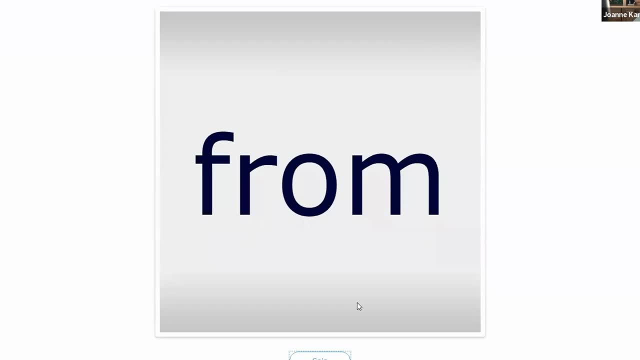 Now we're going on into a sight word game. So we're going to take those words and I put them into a board game. I'm going to have the kids spin the word, read the word and then they get to spin a dice. 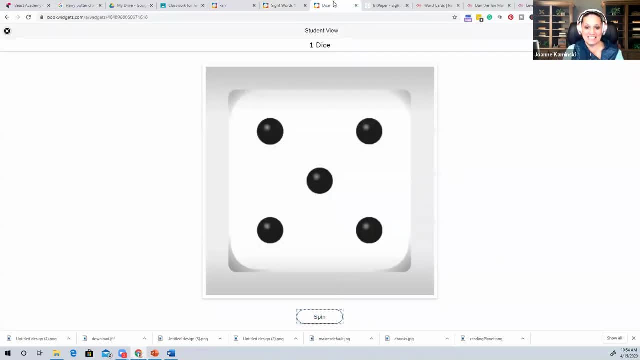 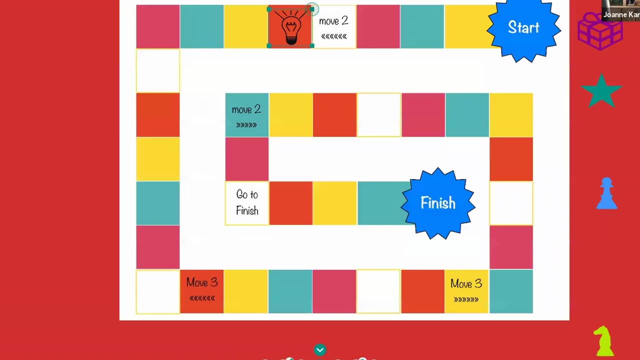 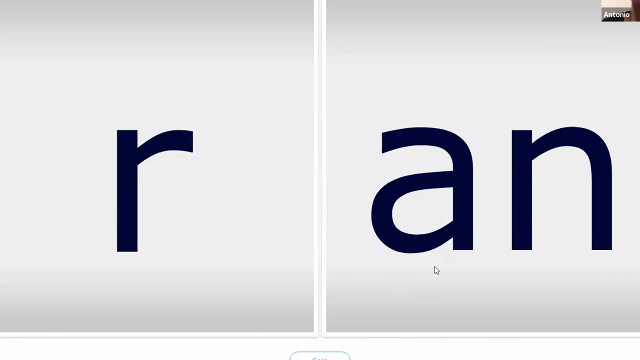 Help. Excellent. Now spin the dice Three. We get to move three places on the board, So we're going to go one, two and three. After the sight words we did rhyme words: R-I-M-E. That's where you have words that end the same but they have a different beginning. 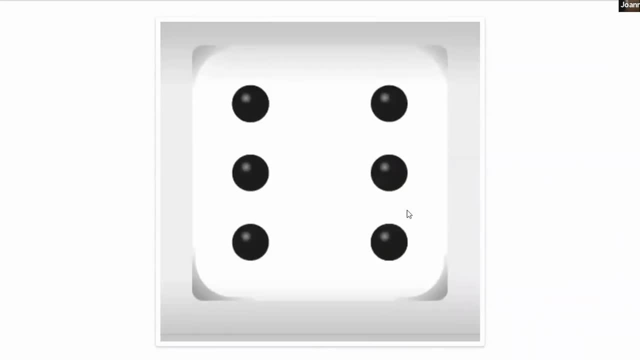 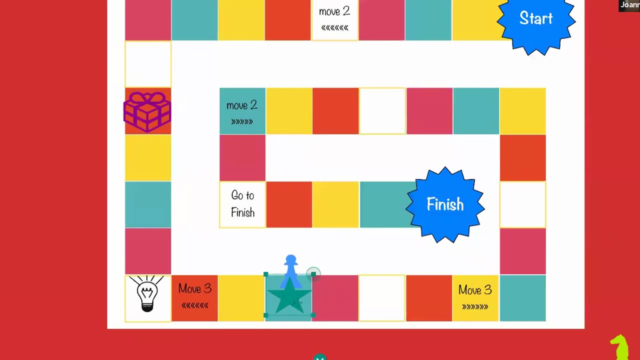 And we use the book widgets tool randomized And we use the book widgets tool randomized to be able to come up with that. Then I had them roll the dice and we were able to move. Now these were also the words that we were going to be learning inside of the book that we were going to that we were going to be introduced to next. 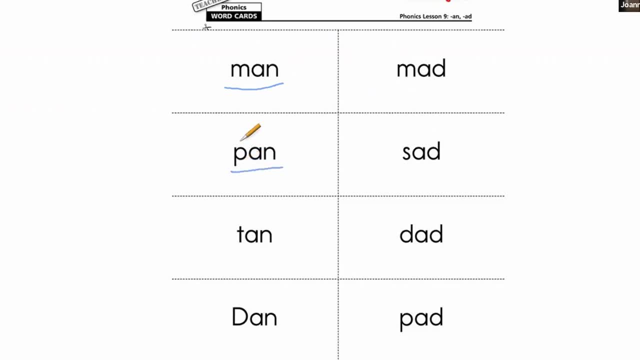 Man Good, What is this word? Pan Pan, Pan, Pan. Good, What is this word? Pan Pan Pan. Yeah, Do you notice something, you guys? Dan Dan Dan is my name. What do you notice about all of these words? 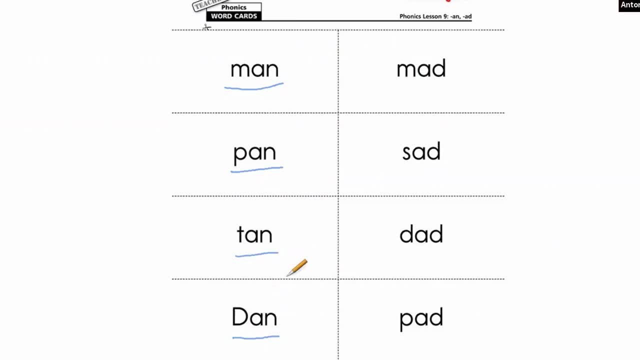 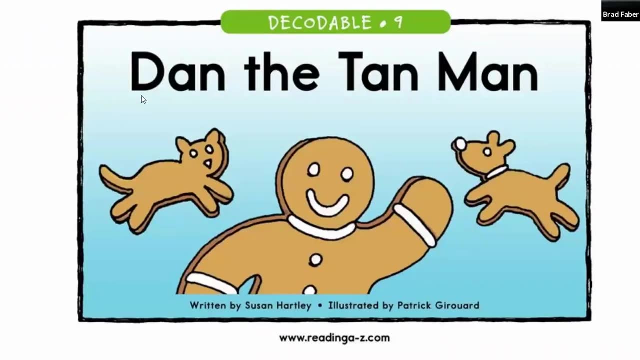 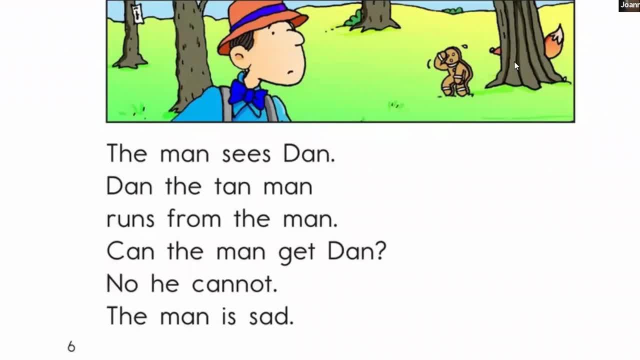 Man, Man, Man, Man. So the title is Dan. All right, Let me unmute you here. Here we go. The man sees Dan, Dan. the tan man runs from the man. Can the man run? Can the man run? 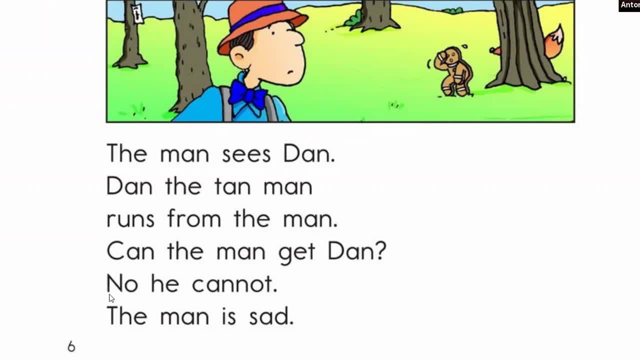 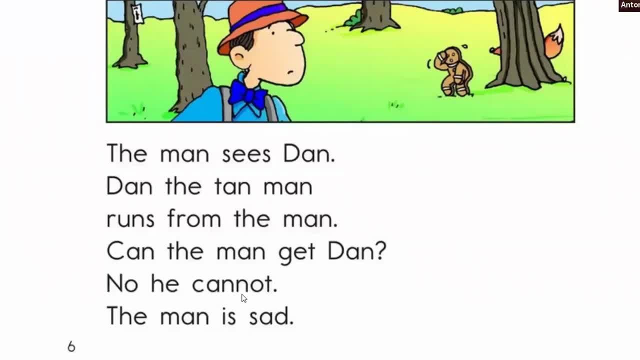 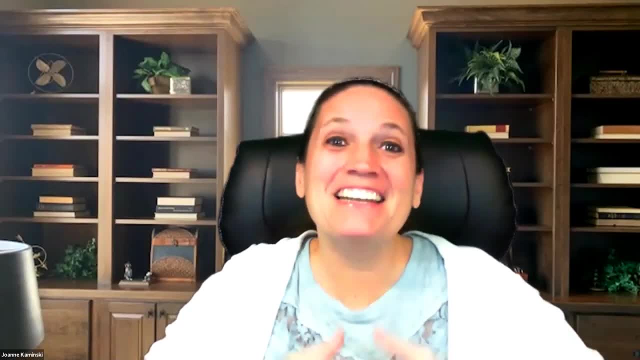 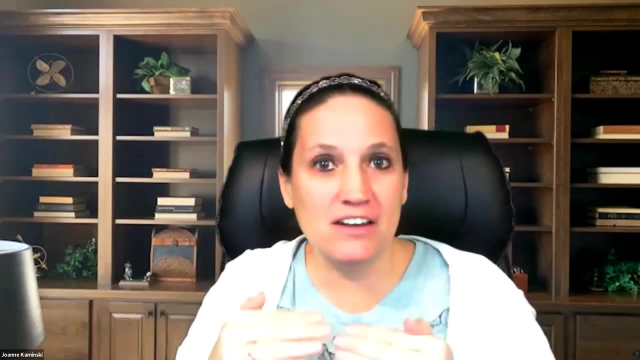 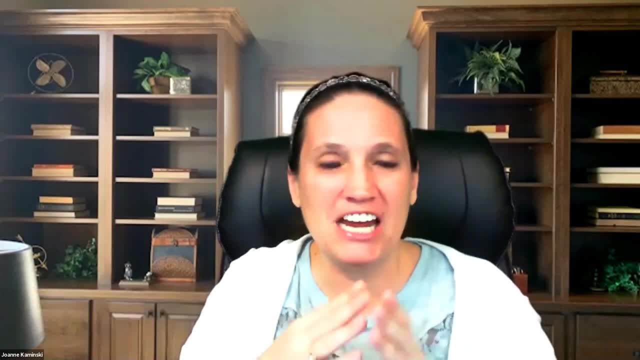 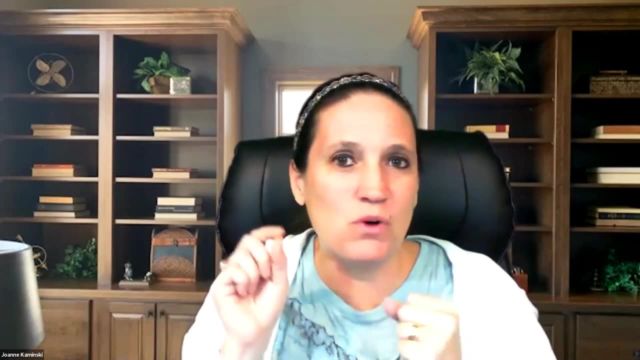 But overall I'm really pleased with how it ended up working and how I figured out little things to really make it work better. So when kids are reading they just kind of want to all read at the same time. but they were all over the place. 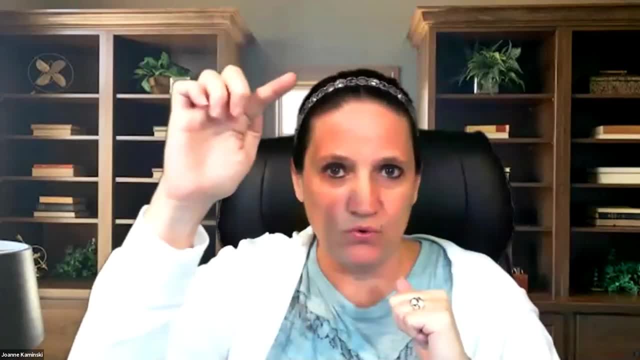 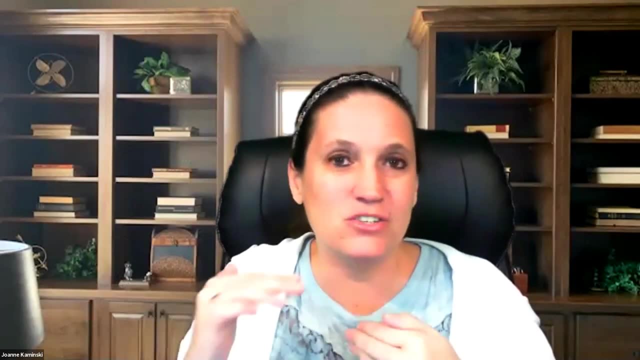 And so what I ended up doing is muting all of the students, only having one kid that was on and the rest of the students were reading along, and it didn't distract the kid that was reading, And so he could read in silence and focus just on figuring out the words. 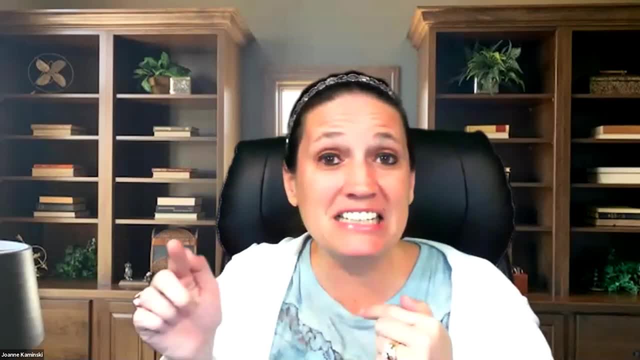 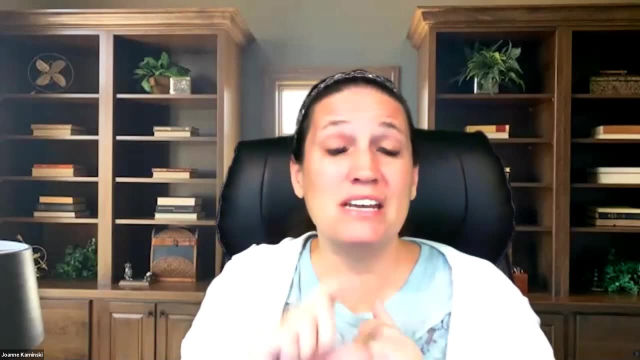 The other kids were reading along as well, And I was able to listen to every single one of them. Then they broke out into their groups and then they read the book with their partner And then we came on back into the big group. It was a lot of fun being able to play the game. 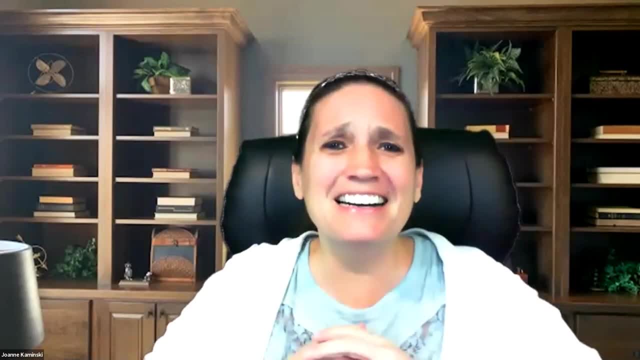 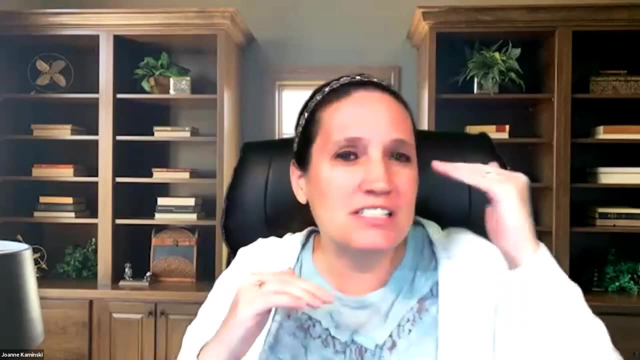 And I realized we're going to make that game go a lot quicker. But this is the wonderful thing about tutoring online and being a teacher: right? You assess all the time. You're thinking, okay, what worked, What didn't work. 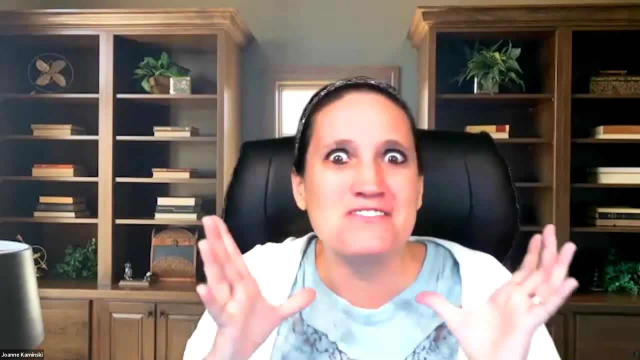 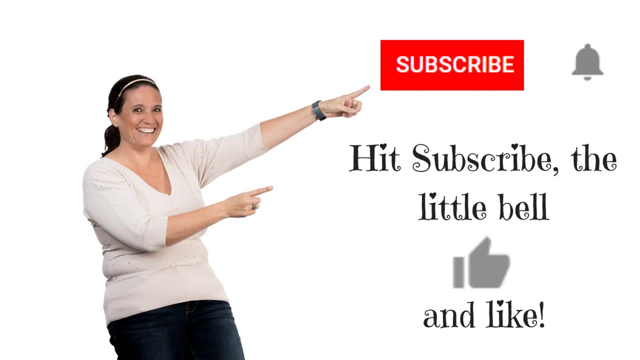 What do I need to change? What do I need to do differently? This is the part that excites me as a teacher: To figure out. okay, how are we going to make this work with these specific kids? And it's a lot of fun. 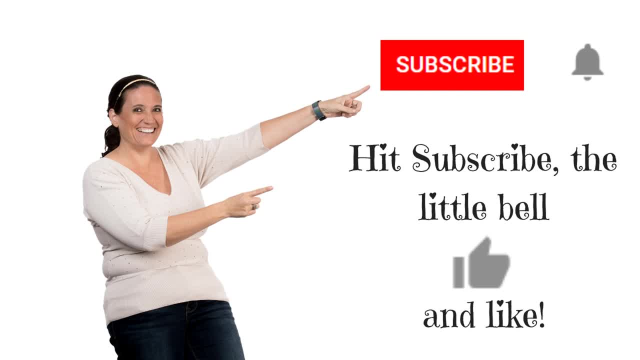 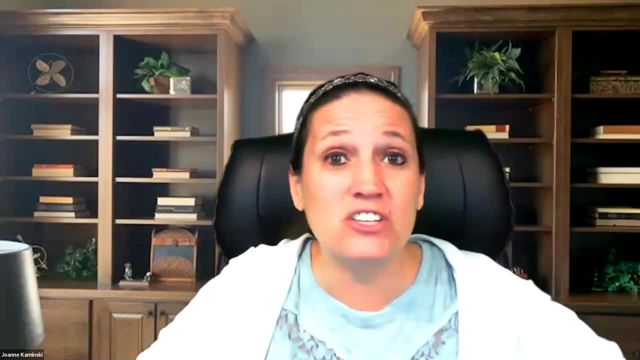 And if you like seeing videos like this that can help you with being able to run your online tutoring business, please hit that like and that subscribe button And if you have any ideas for any videos that you'd like to see in the future, comment below. 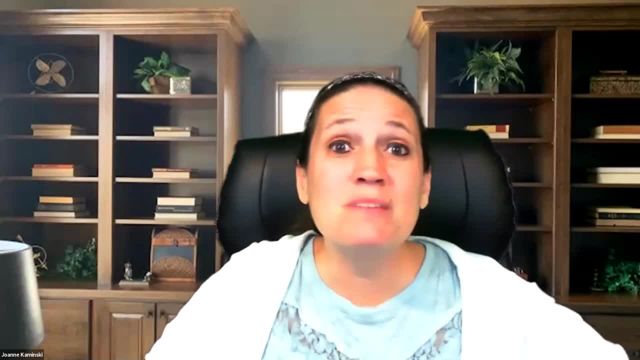 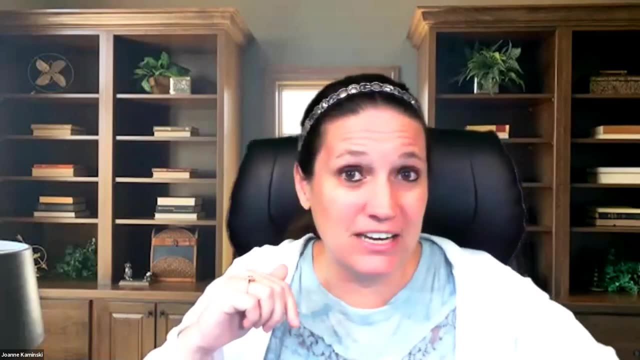 I'd love to be able to hear what you would like to see Now. I'm going to give you a more in-depth training on RISED Kids. Now, before I share with you where you can get that specific video, I'm doing a free. 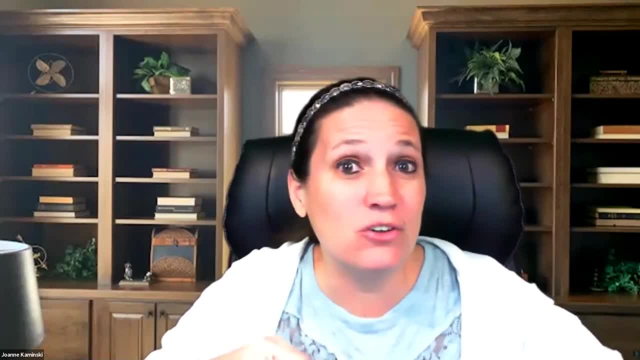 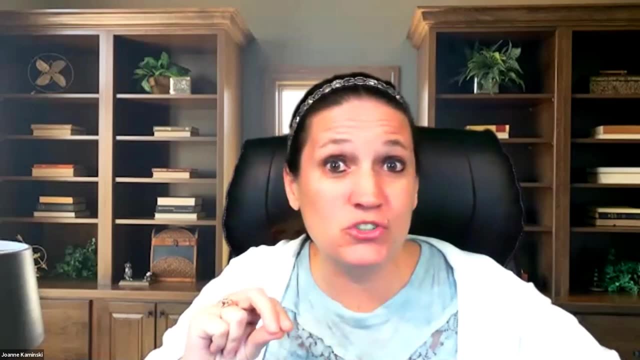 training next week. Next week you're going to get to learn how I close the reading gap- a full year with 8 to 12 hours of instruction. So if that is something that you are interested in doing with your students, definitely come join me. 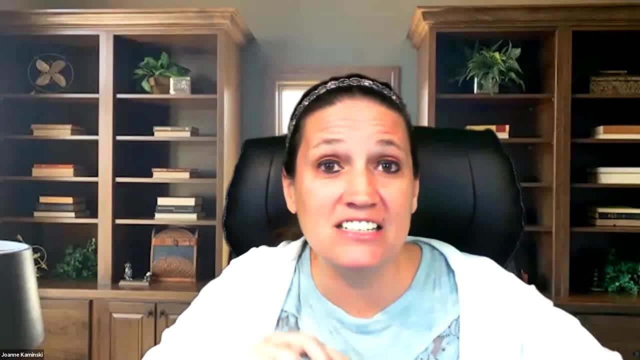 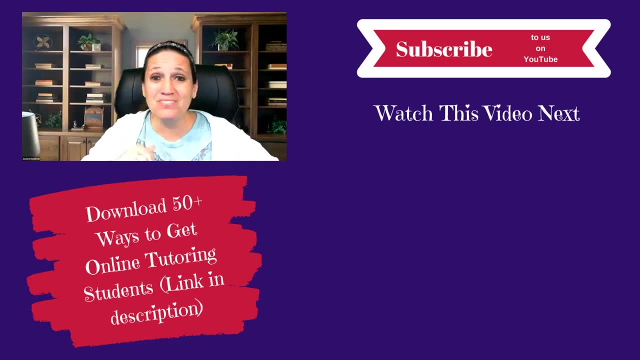 I'm putting the link inside of the description. All you have to do is click that description, click that link and sign up so that you can be informed when that is And to see the video on all of the features of Kids A to Z, so that you can use that amazing. 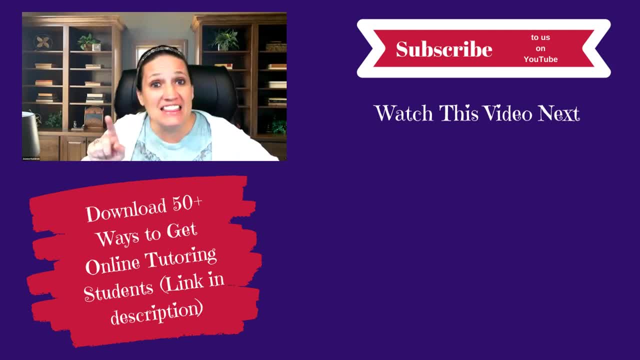 tool with your students, then you're going to want to stick around, hit that video that's on the right-hand side so that you will be able to watch it and see if it could be a good tool for you to be able to use with your students.